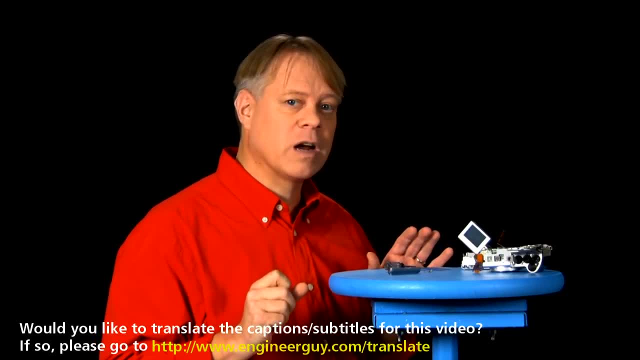 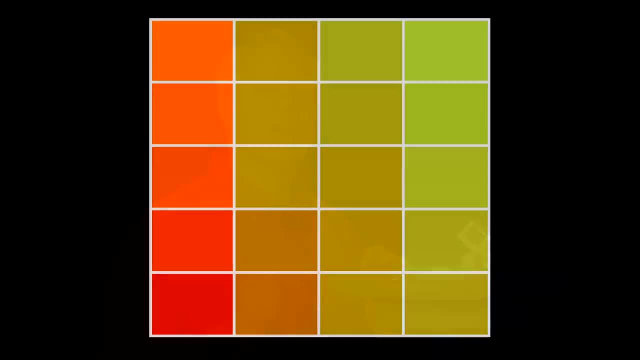 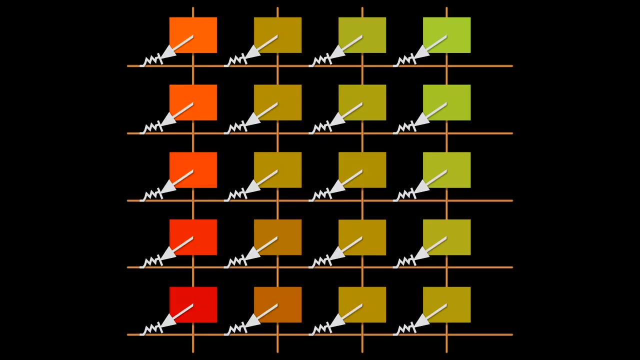 Now, the key to understanding how digital photography became cheap and ubiquitous lies in the ingenious way that the CCD transfers the image into the camera's memory. The easiest and most straightforward way would be to use wires to connect each pixel in an XY grid, But that presents a problem. Here's what goes wrong. 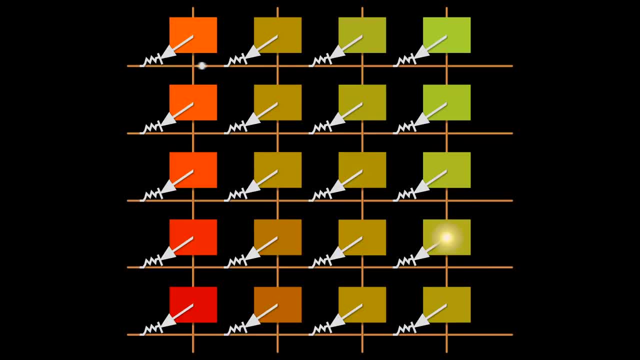 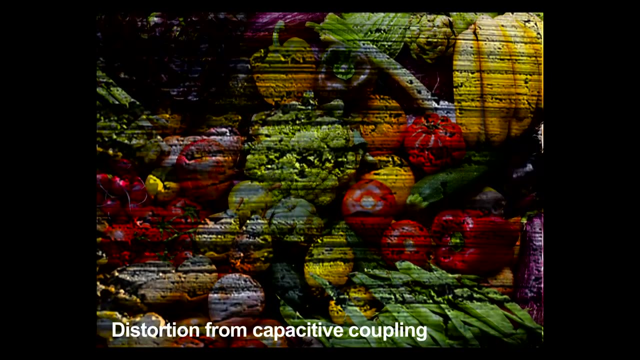 After exposing the grid to light, we can use these wires to capture the image. We have to read the information pixel by pixel, measuring the charge on each section of the grid. This makes sense in principle, except all of the pixels and their electronic components leak a small bit of charge that distorts the charge coming from each pixel and leads to striations and patterns in the image. 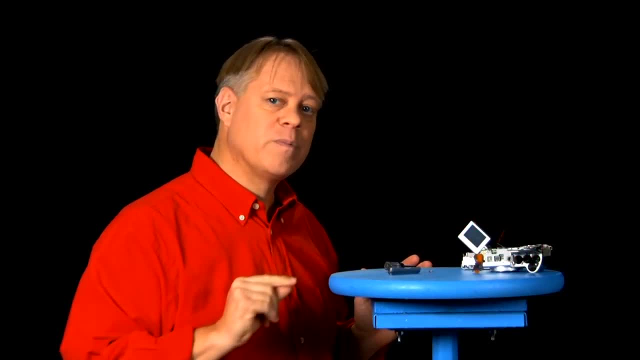 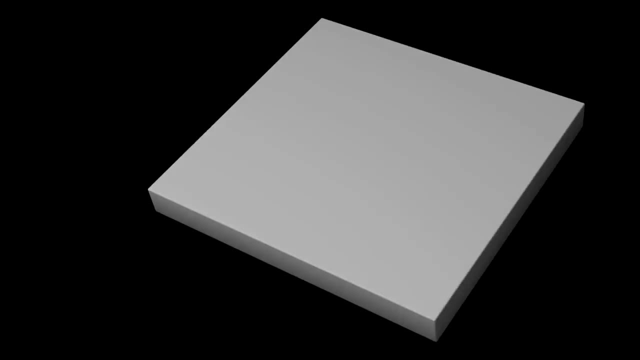 This distortion, called capacitive coupling, increases as the number of pixels increases. A CCD solves this problem in a very simple way. The pixels have no wires attached to them. A CCD is made from a slab of silicon. To make each pixel within the slab, engineers create insulating sections called channel stops. These divide the slab into rows. 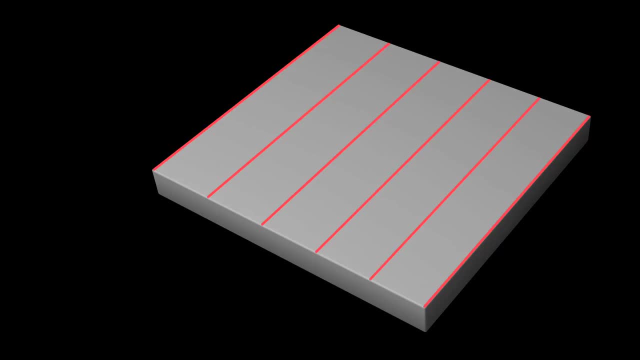 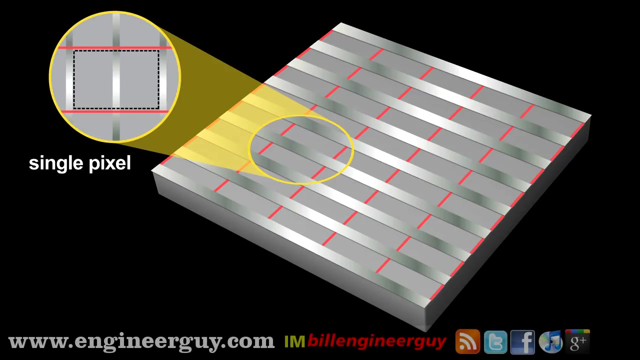 The surface is covered with a thin layer of insulating silicon dioxide and then, perpendicular to the channel stops, engineers deposit thin strips of metal, typically aluminum. Each pixel, then, is one section bounded by channel stops and aluminum. So now we have our grid of pixels. Recall that when light strikes the whole array, the silicon pixels build up charge proportional to the intensity of the light's charge. 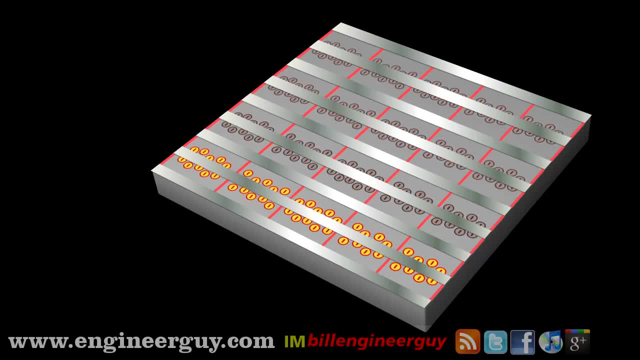 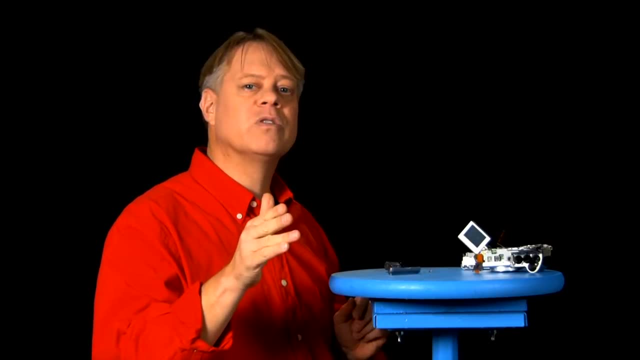 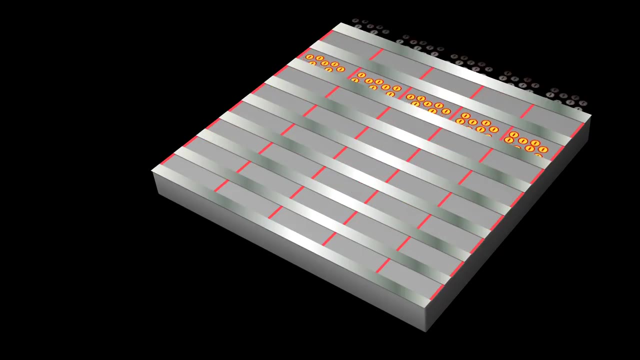 We then have a captured image stored as charge within each pixel. The great innovation of the CCD was how it moved the image from the silicon array to the camera's memory system without using external wires that would distort the image. The CCD shifts the charges from row to row without wires, until they reach the bottom when a readout register transfers the charge to the camera's memory with very little distortion. 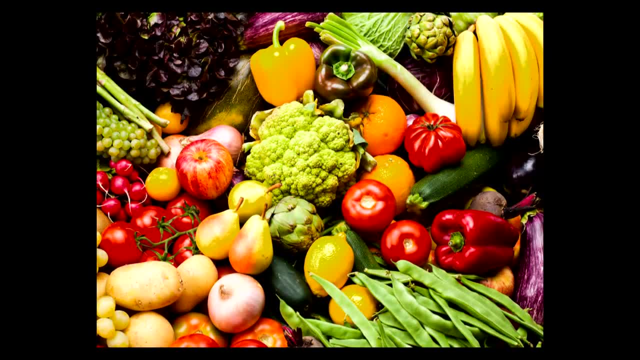 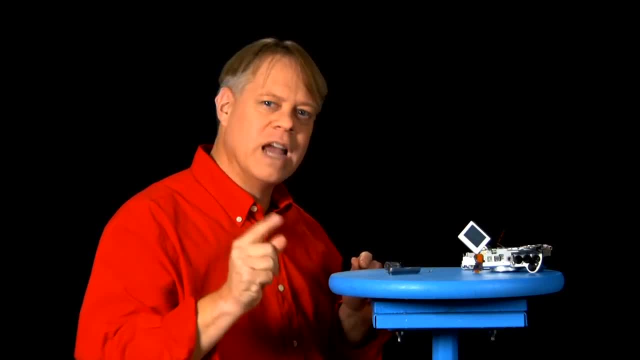 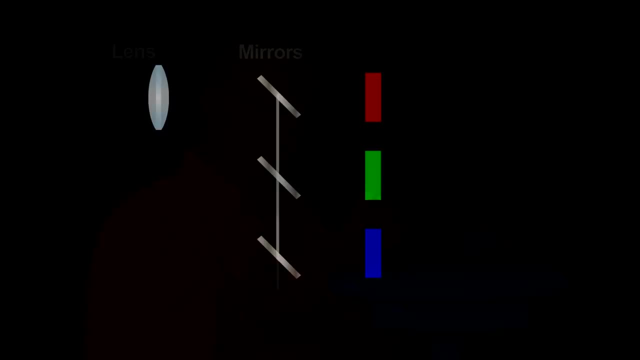 The camera then counts the charges and constructs the image using that data. Now one last important question: How do we get color? A CCD only detects total light intensity, which is useful for producing a black and white image, But for a color photograph we need to separate the entering light into red, green and blue. 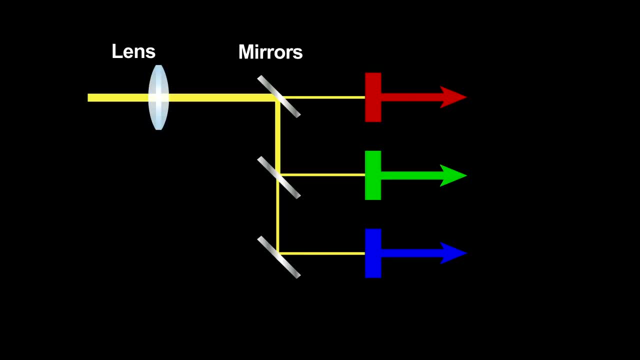 The most obvious solution is to filter the light into those three colors using three separate CCDs to capture red, blue and green information and combine them into a full color image. However, engineers have created a cheaper solution. Instead of using three separate CCDs, they use a little math, so they only need one.